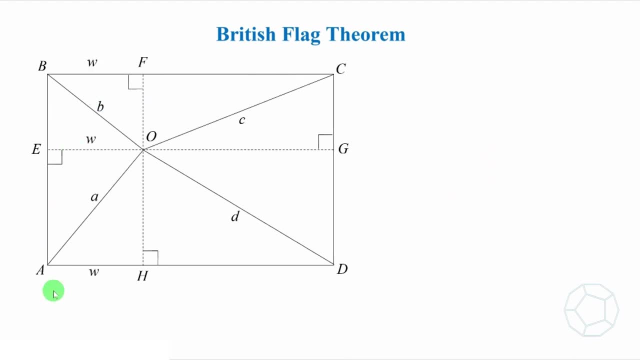 For convenience let's label the lengths of the sides as W, X, Y and Z. Then we can apply Pierre Frekal's theorem in four triangles. In triangle OAE, W square plus X squared is one square is equal to a square. Let's call this equation 1.. In triangle OBF, w square plus y square is equal. 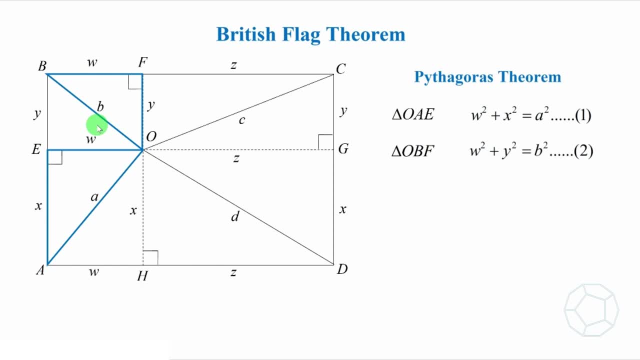 to b square. Let's call this equation 2.. Likewise, in triangle OCG, y square plus z square is equal to c square. We call this equation 3.. Lastly, in triangle ODH, x square plus z square is equal to. 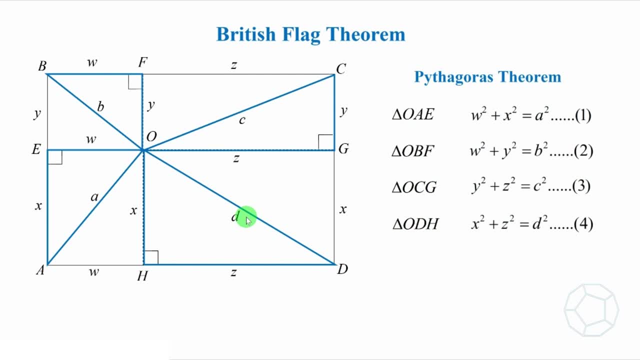 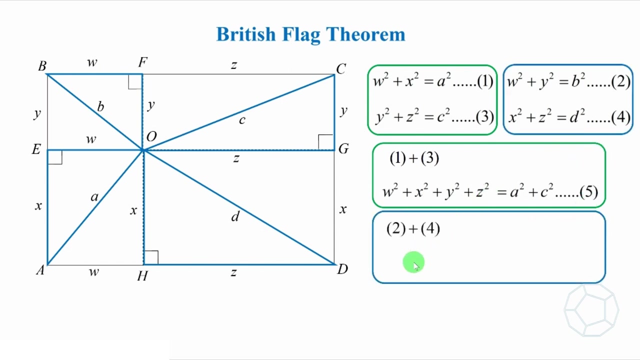 d square. Let's call this equation 4.. Can you see any pattern behind? Let's add up equation 1 and equation 3.. Then we have w square plus x square plus y square plus z square is equal to a square plus c square. We call this equation 5.. We do the same for equation 2 and equation 4.. Therefore, 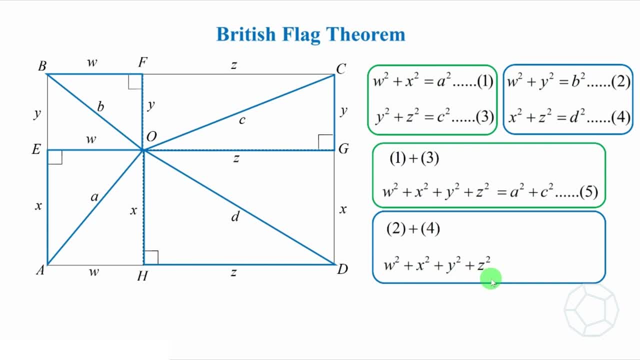 w square plus x square plus y square plus z square is equal to b square plus d square. Let's call this equation 6.. Comparing these two equations, the left-hand side are the same, So the right-hand side should be equal, That is a square plus c. 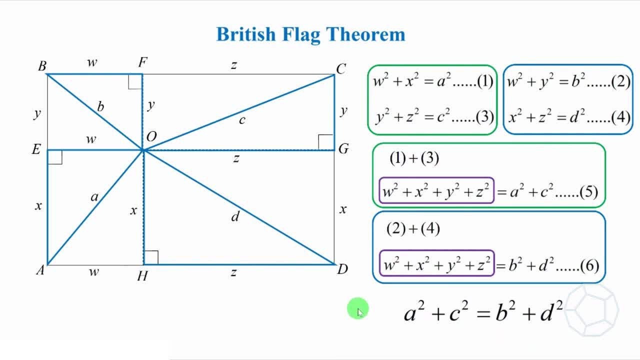 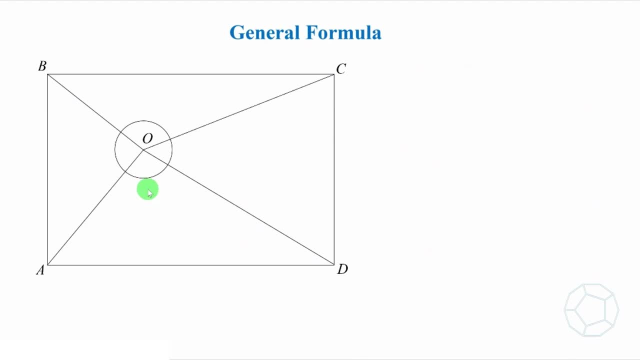 square is equal to b square plus d square. This completes the proof of the theorem. Now we go back to our original problem. We use the letters a, prime, b, prime, c, prime and d prime to solve the problem. We use the letters a, prime, b, prime, c, prime and d prime to solve the problem. 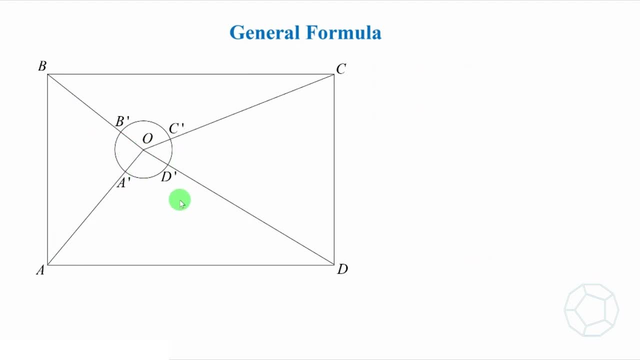 To denote the points of intersection of the line segments and the circle, Let the lengths of line segment outside the circle be a prime, b prime, c prime and d prime. The radius of a circle is r. Using the same notation of a, b, c and d, we have: a is equal to a prime plus r.